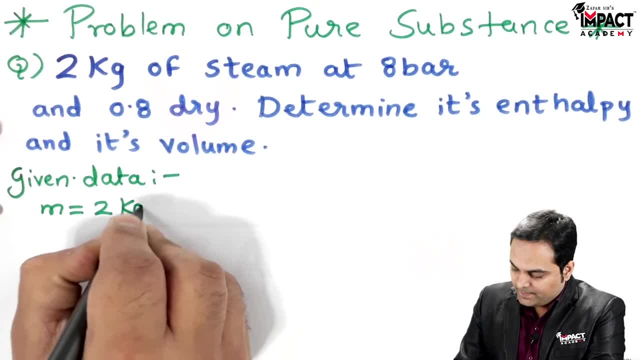 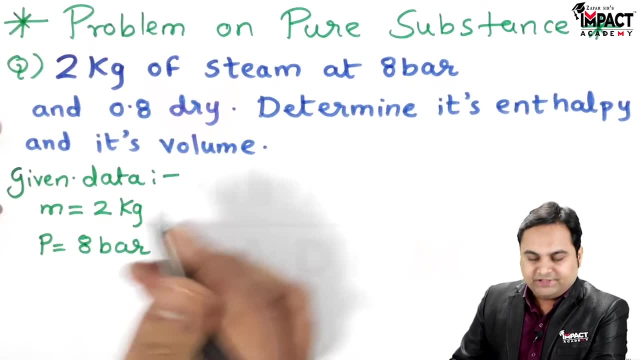 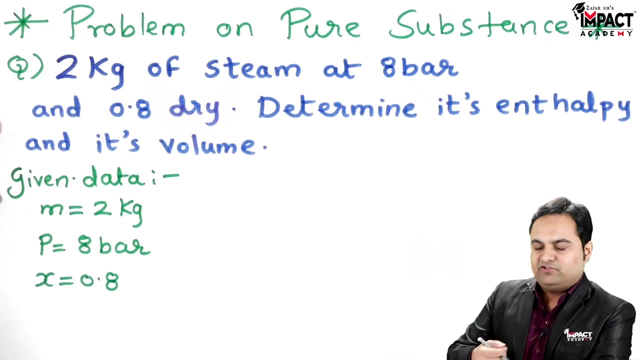 So the mass of steam is given as 2 kg At 8 bar pressure of the steam is given And 0.8 dry. that is the dryness fraction. It means it is 80% dry and 20% wet, which means 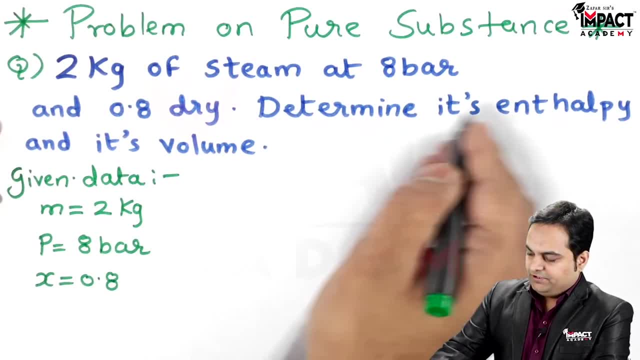 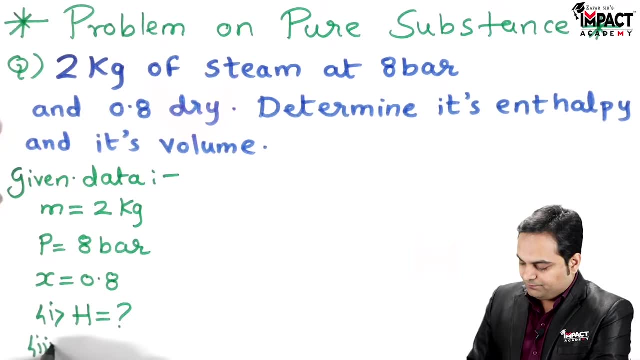 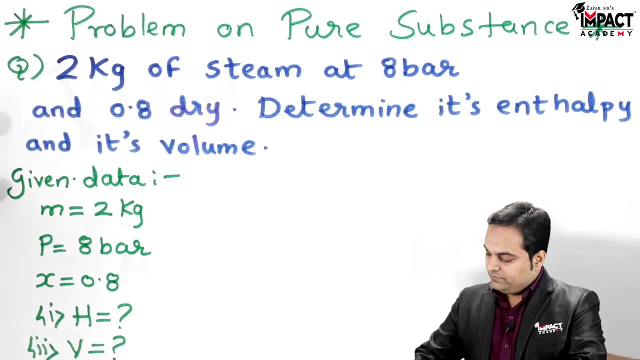 it contains 20% moisture or water vapor Determine its enthalpy and its volume. So we have to find out the total enthalpy and the total volume of this steam. Now I'll write the solution here itself, that when I'm solving this problem. 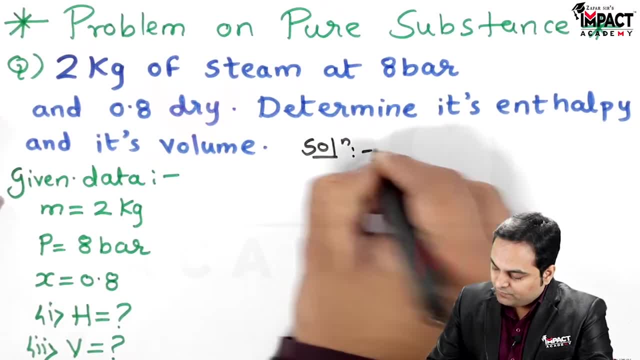 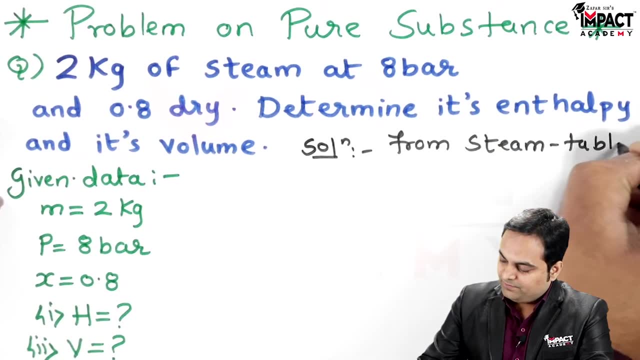 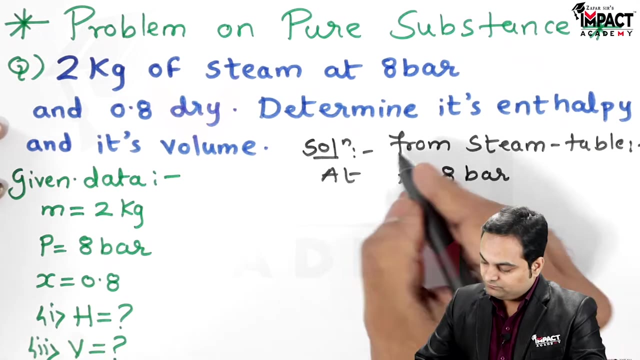 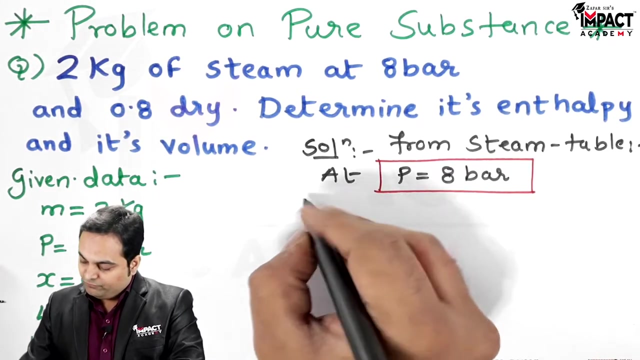 into the solution. part First, from steam table, because I'm going to use the steam table over here. From steam table corresponding to a pressure of 8 bar. Now, at pressure of 8 bar in the steam table I'm going to find HF value, that is, the enthalpy of saturated liquid. 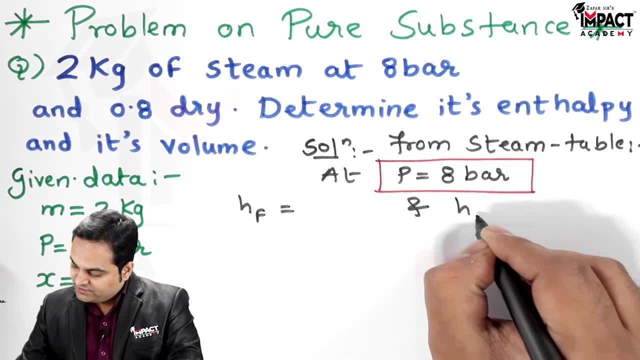 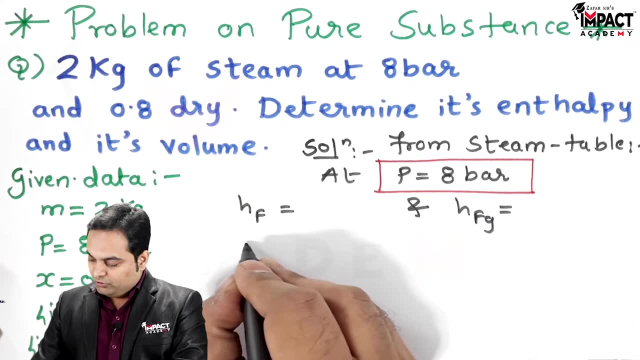 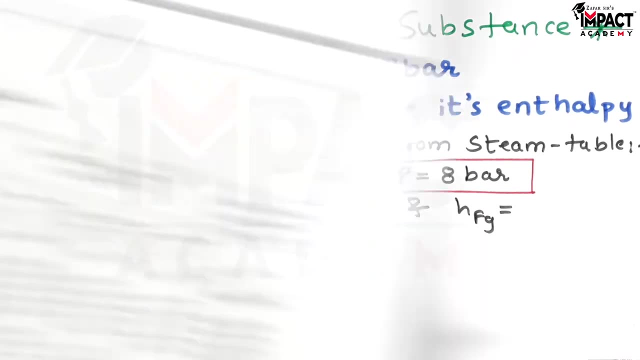 Then also I'm going to find HFG, the latent enthalpy, And since volume is asked, I'm going to get the volume of the dry vapor corresponding to 8 bar pressure, because that would be required in the problem. So go into the steam table And in the steam table the table number 2 is 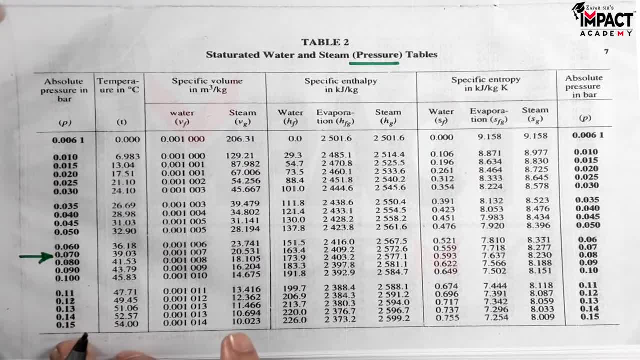 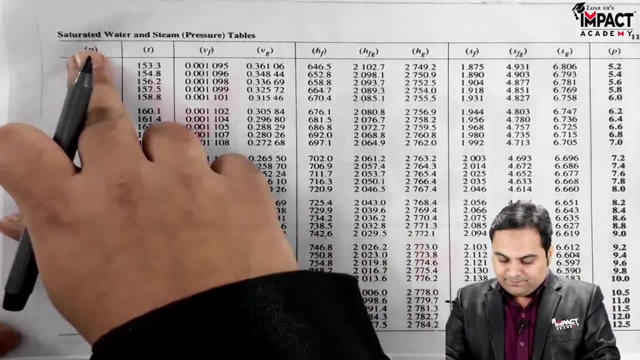 the pressure table. Go for the pressure, Which pressure is given. It is given as 8 bar, So going up to the pressure of 8 bar. So in the steam table at a pressure of 8 bar, as I can see here, there is a pressure of 8 bar. 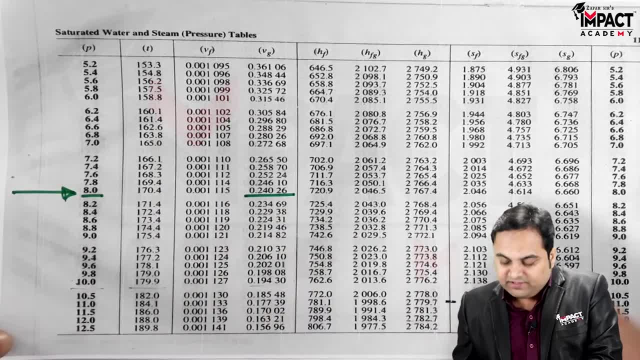 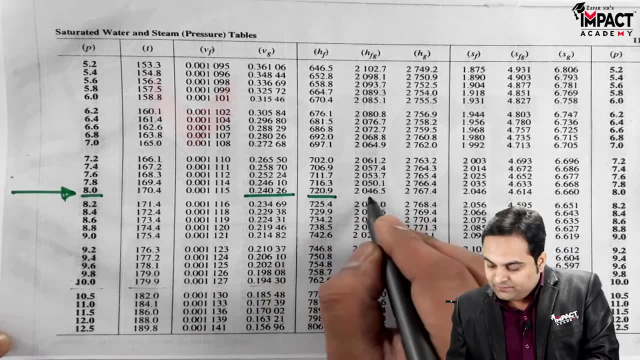 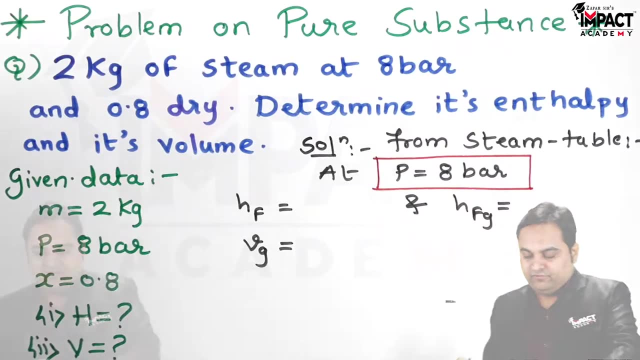 Corresponding to this. take the values of VG, that is the specific volume of the dry vapor. HF, it is the enthalpy of the saturated liquid, And HFG latent enthalpy. Take these three values from pressure of 8 bar. So I'm writing these three values. 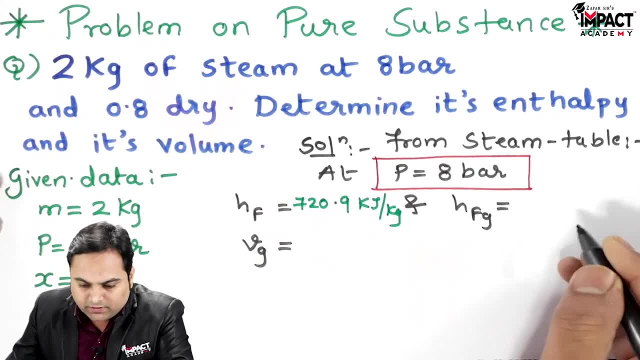 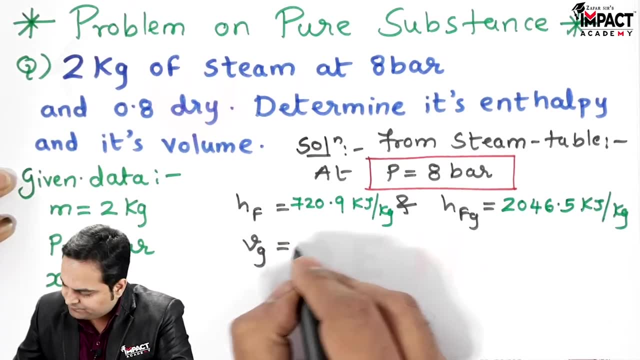 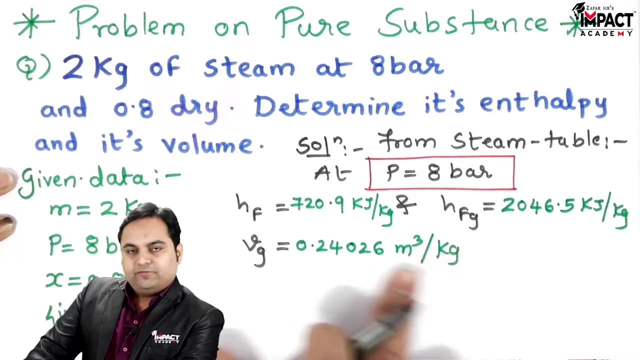 Retail quantity: 2400, 2012.904.. So that is 720.904 kilojoules per kg, HFG 2046.5 And VG value后 Hard pressure and главное Amount, Specific volume. since the value is specific, it means it is based on per kg. So the unit 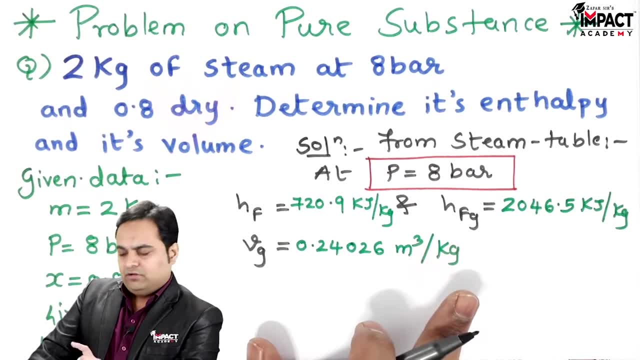 is meter cube per kg And the entire steam table is based upon specific properties, that is, taking the quantity of steam as 1 kg. Now I'll say that, therefore, the enthalpy of wet steaming is based on a per kg result And 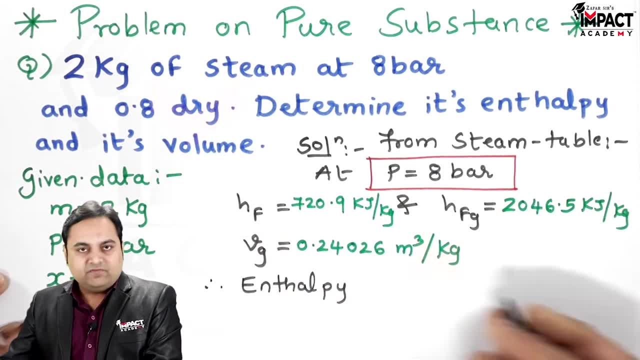 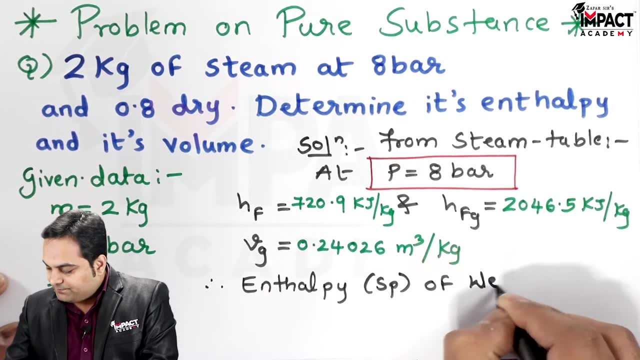 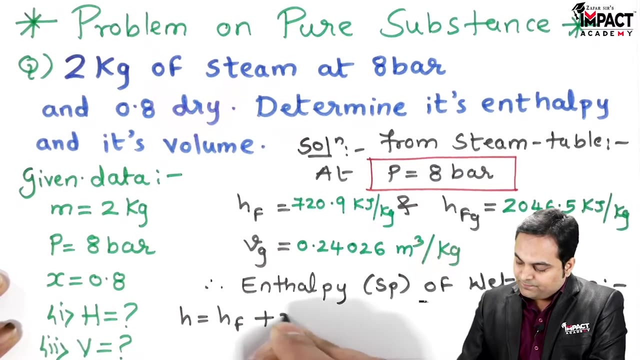 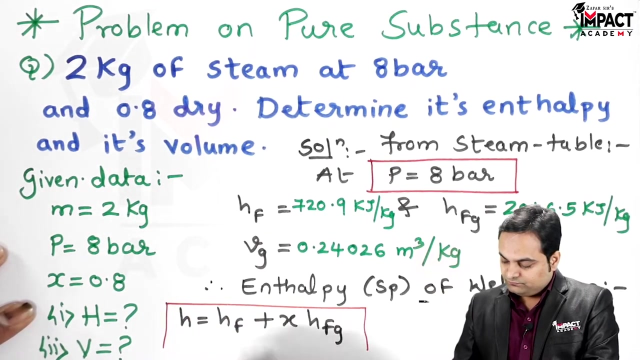 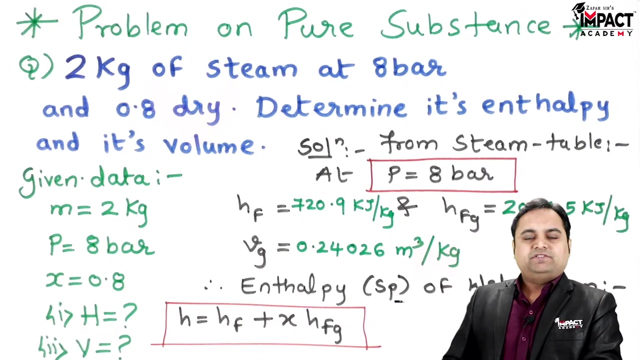 stream and the enthalpy which I am finding here. that is the specific enthalpy first. so enthalpy, specific enthalpy of wet stream. it is small, h is equal to the formula is hf plus x into hfg. and to refer this formula I would be providing the link of the formula list in the description. 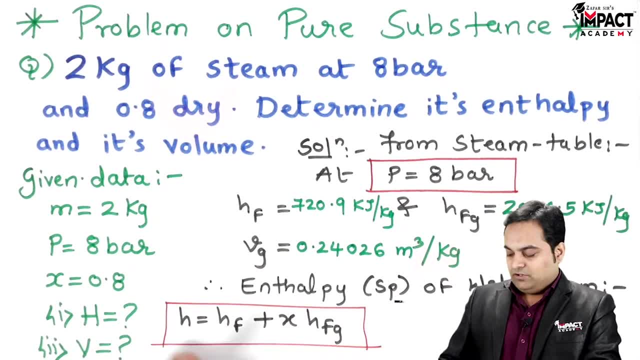 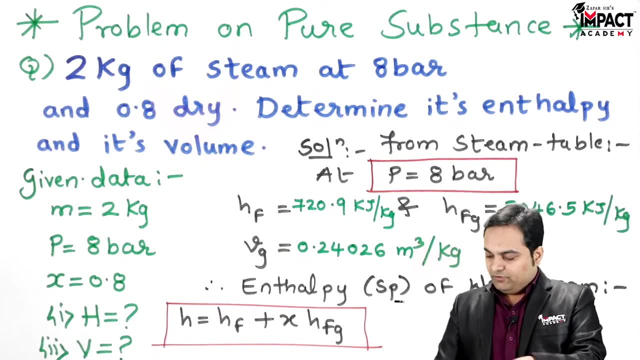 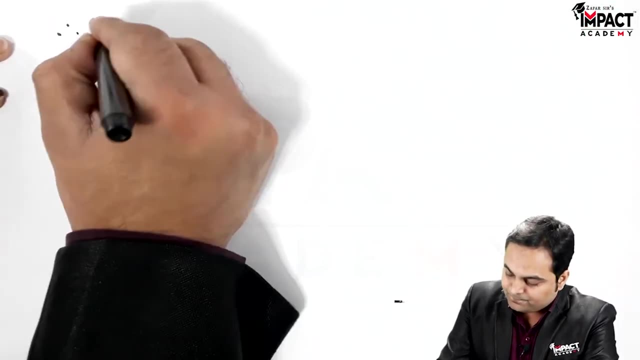 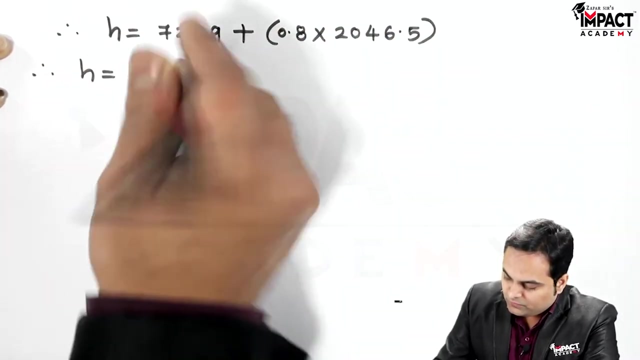 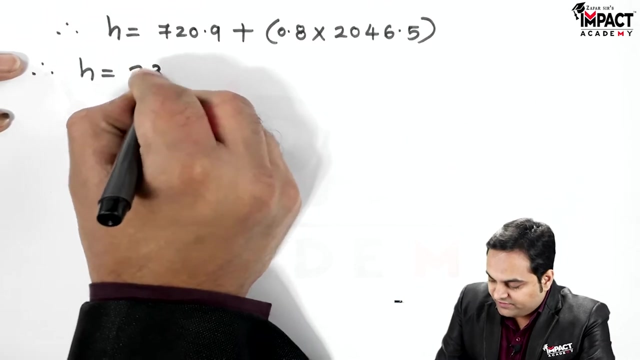 below, so that you can just see that how this formula comes from. that is the fe, we can say the enthalpy of the wet stream. now, putting the values of hf, x, the dryness fraction in hfg, I will get small h here. so on calculating this, the specific enthalpy comes out to be: it is 2358.1. 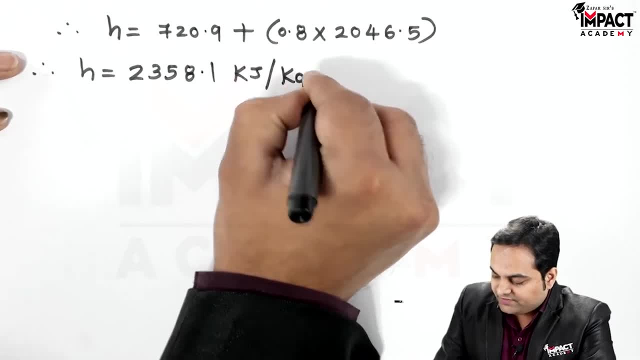 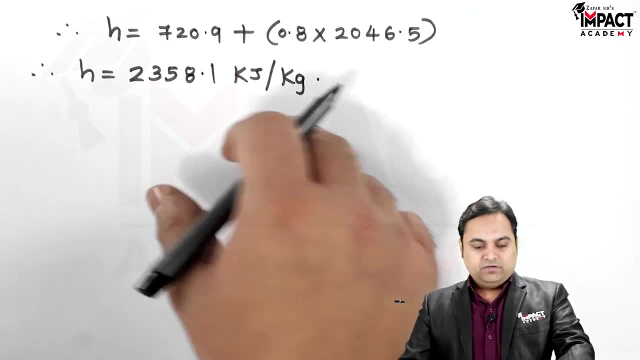 kilojoule per kg. so that is the specific enthalpy. if in this problem mass was not given, then this would have been the answer. but since the mass is given, it is 2 kg, so that is the specific enthalpy. now, on calculating this in 2 individuals, 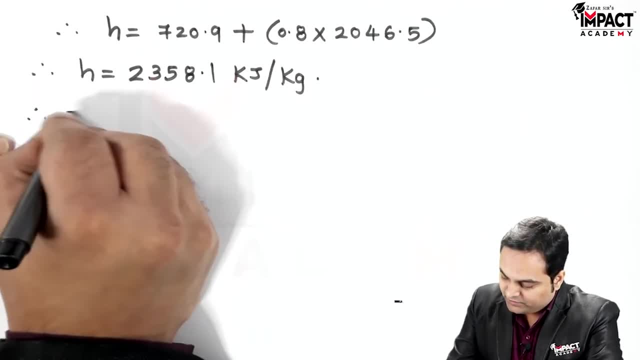 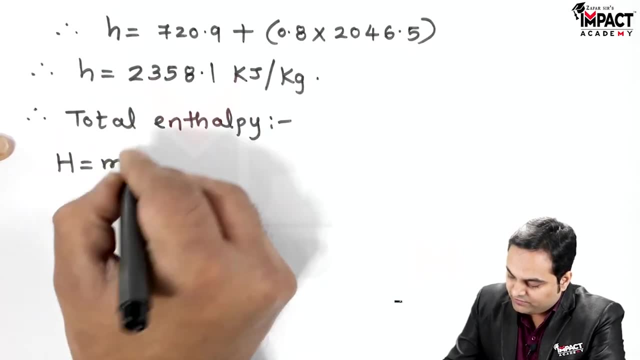 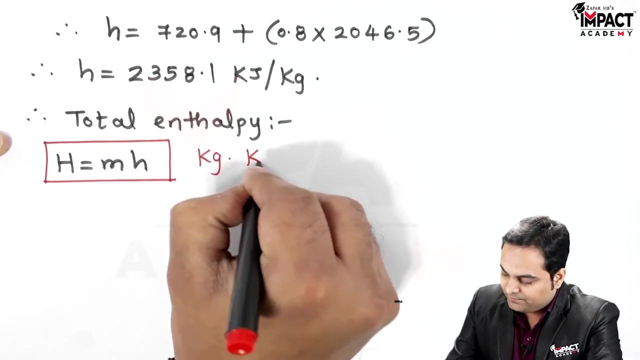 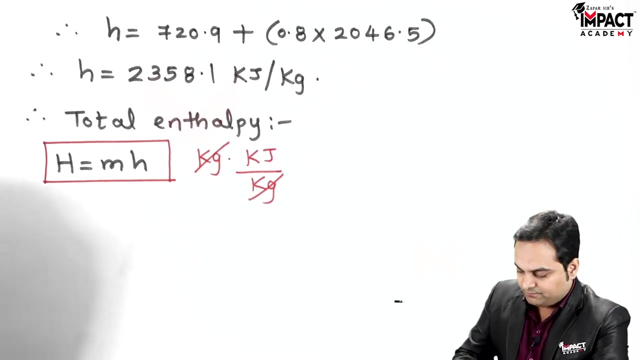 so one of these 41 concerted number means k, g, so I have to get the total enthalpy, which is capital H. so therefore total and El bi is given by x. the enthalpy with mass mass is IN terms of kg enthalpy, kilojoule per kg. so kg in kg will. 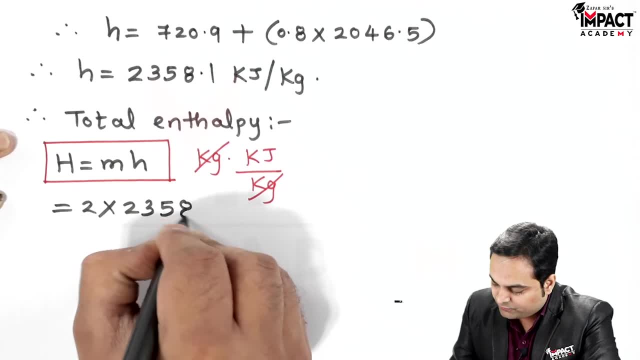 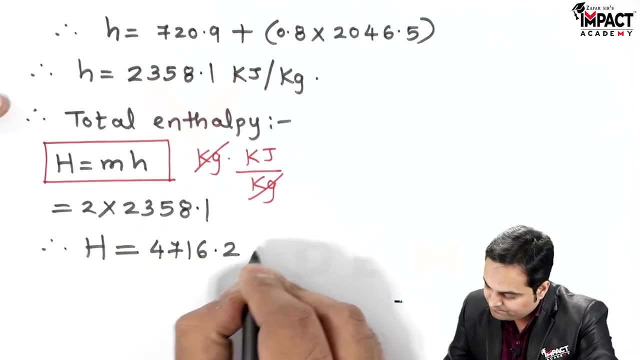 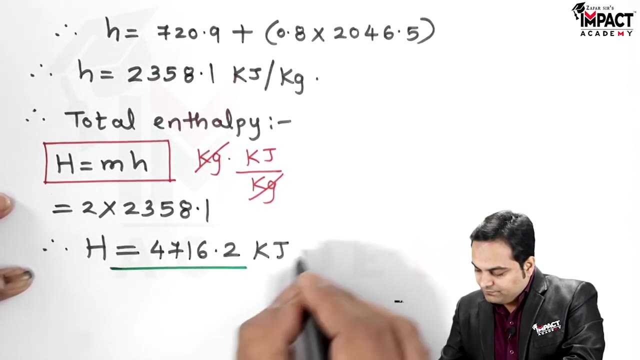 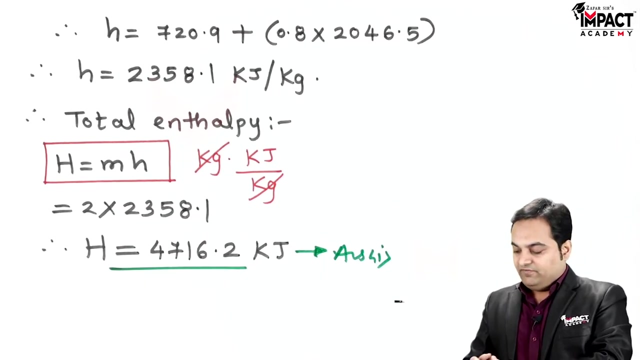 two into two, three, five, eight point one. so capital H value will be. so it is four thousand seven hundred and sixteen point two kilojoule, and that's the first answer. that's the total enthalpy of the given steam. next, to get the total volume of the stream, first I'll find the specific volume. so